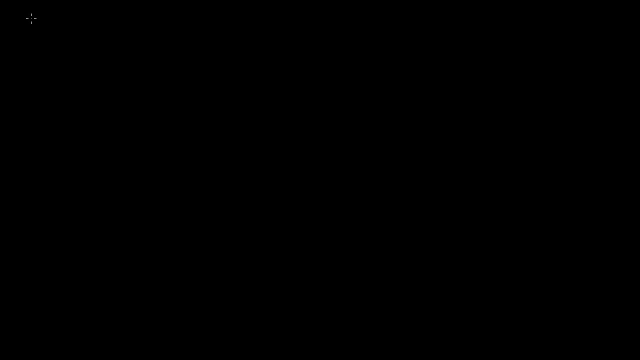 In the last video we learned what it meant to take the product of two matrices. So if we have one matrix A and it's an m by n matrix and then we have some other matrix B, let's say that's an n by k. 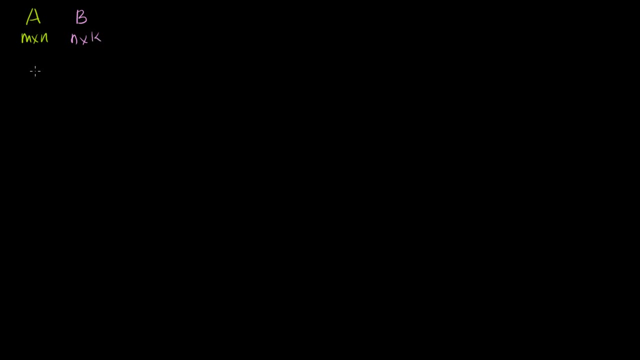 matrix, then we've defined the product of A and B to be equal to. and actually, before I define the product, let me just write B out as just a collection of column vectors, So we know that B can be written as a column vector B1,. 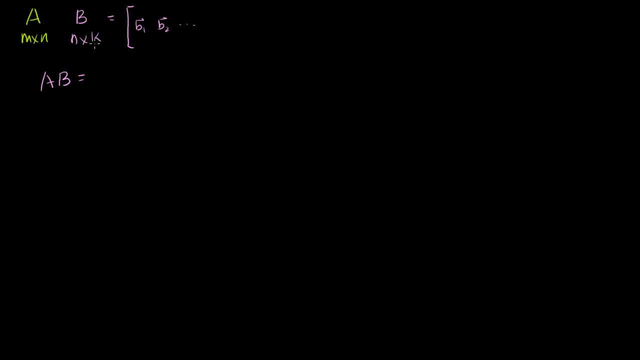 another column, vector B2, and all the way it's going to have k of them because it has exactly k columns, So Bk. So in the last video we defined the product of A and B and they have to have the columns of A, have to be the 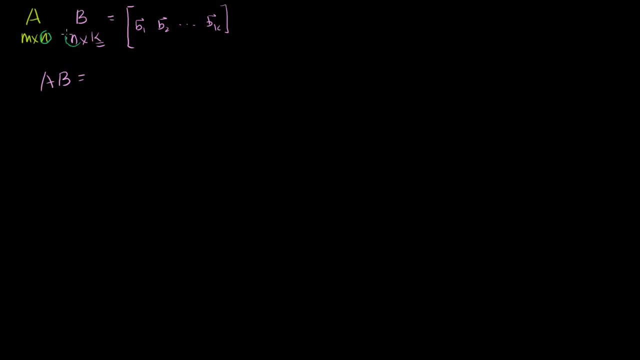 same as the rows of B in order for this to be well-defined. But we defined this product to be equal to A times each of the column vectors of B, So it's equal to. let me switch back to that color. it's equal. 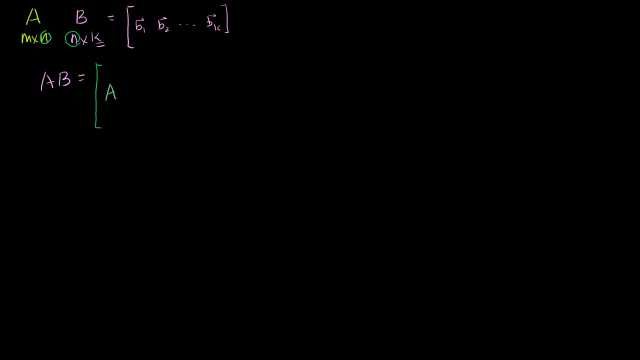 to A times. let me do it in the color that I did it: A times B1.. And then the second column of our product is going to be A times B2.. Our third product is going to be A times B3.. B3, all the way to A times Bk, right there. 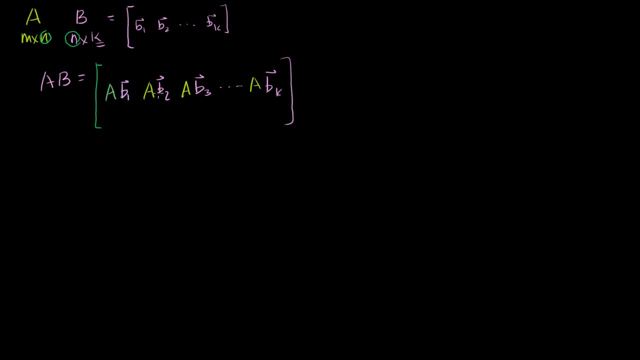 And the whole motivation for this. you've probably seen this before, maybe in your Algebra 2 class. It might have not been defined exactly this way, but this is equivalent to what you probably saw in your Algebra 2 class. But the neat thing about this definition is that the 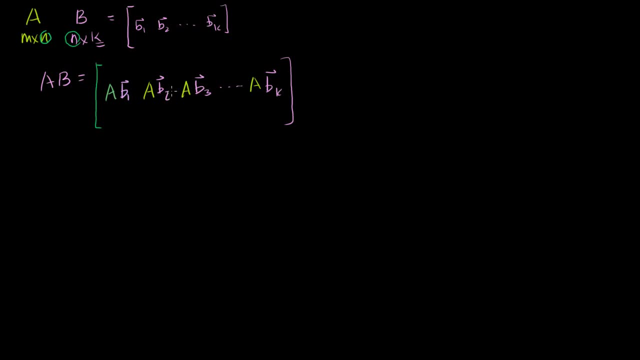 motivation came from the composition of two rows of A's. Let's see what that means: Two linear transformations whose transformation matrices were the matrices A and B, And I showed you that in the last video. With that said, let's actually compute some matrix-matrix. 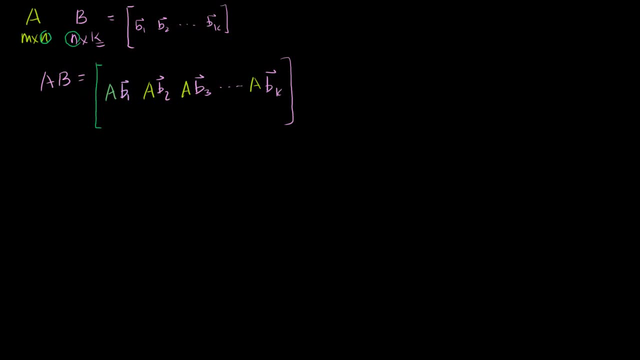 products. just so you get the hang of it. So let's say that I have the matrix A. Let's say that A is equal to the matrix 1, minus 1,, 2,, 0, minus 2, and 1.. 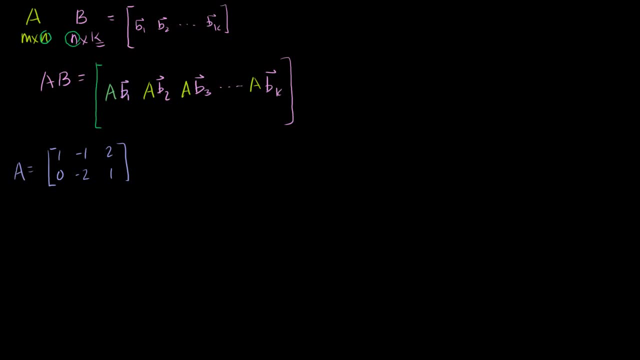 I keep the numbers low to keep our arithmetic fairly straightforward. And let's say that I have the matrix B. Let's say that it is equal to 1, 0, 1, 1, 2, 0, 1, minus 1.. 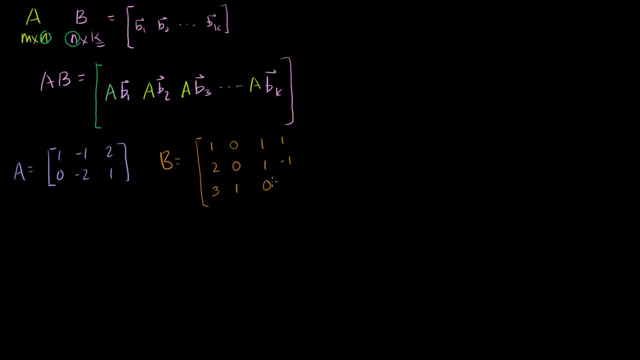 And then 3, 1, 0, 2.. So A is A, 2, 0, 1, minus 1.. 2, 0, 1, minus 1.. 2 by 3 matrix, 2 by 3, 2 rows, 3 columns, and B is a, 3 by 4. 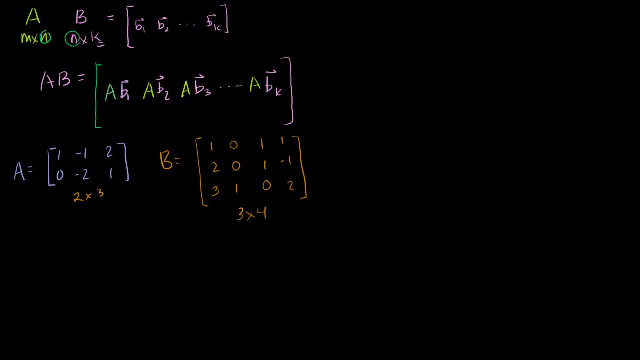 matrix. So, by our definition, what is the product AB going to be equal to? Well, we know it's well-defined, because the number of columns here is equal to the number of rows. So we can actually take these matrix vector products. You'll see that in a second. 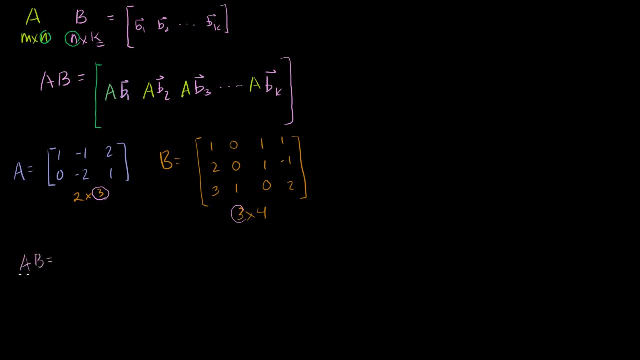 So AB is equal to the matrix A times the column vector 1,, 2,, 3.. That's going to be the first column in our product matrix And the second one is going to be the matrix A times the column 0,, 0,, 1.. 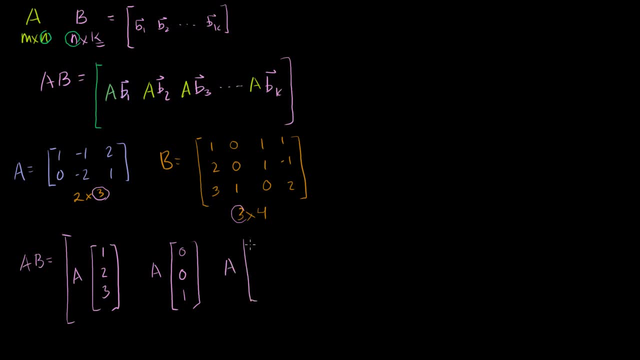 The third column is going to be the matrix A times the column vector 1, 1,, 3.. 0.. And then the fourth column in our product vector is going to be the matrix A times the column vector 1, minus 1,, 2.. 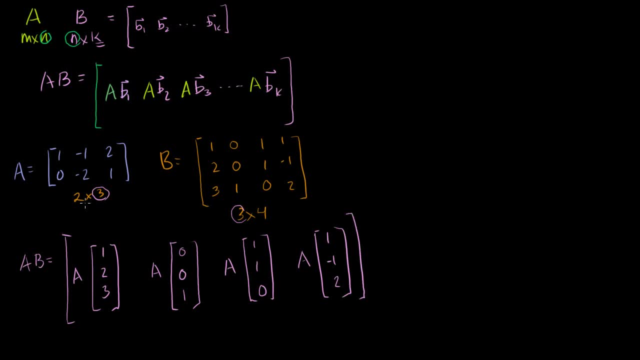 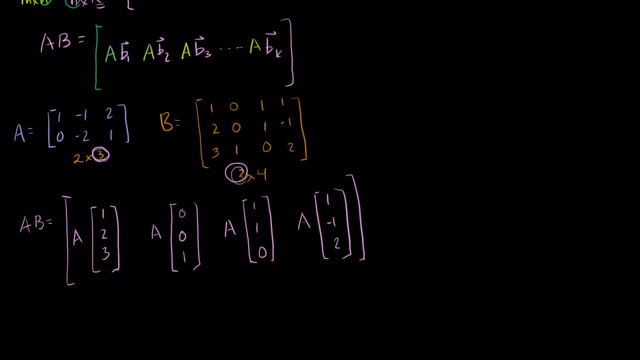 And when we write it like this, it should be clear why this has to be, why the number of columns in A have to be the number of rows in B, Because the column vectors in B are going to have the same number of components as the number of rows in B. 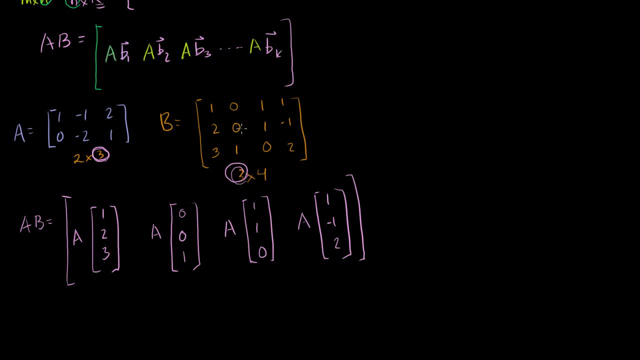 So all of the column vectors in B. So if we call this B1, B2, B3, B4,, all of my Bi's- let me write it this way- all of my Bi's where this i could be 1,. 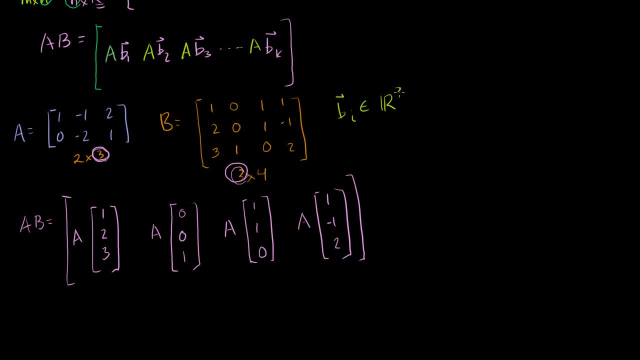 2, or 3, or 4, are all members of R3. So we only have matrix vector products well defined when the number of columns in your matrix are equivalent to, essentially, the dimensionality of your vectors. That's why that number and that number has to be the same. 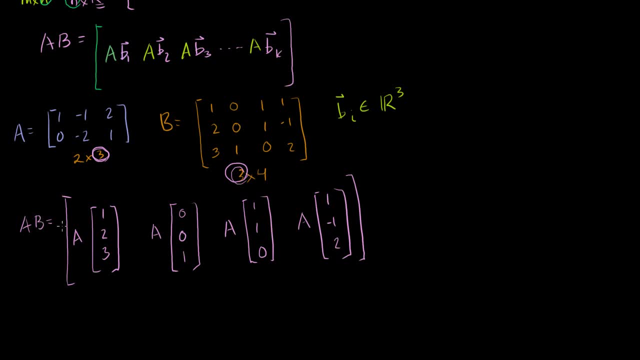 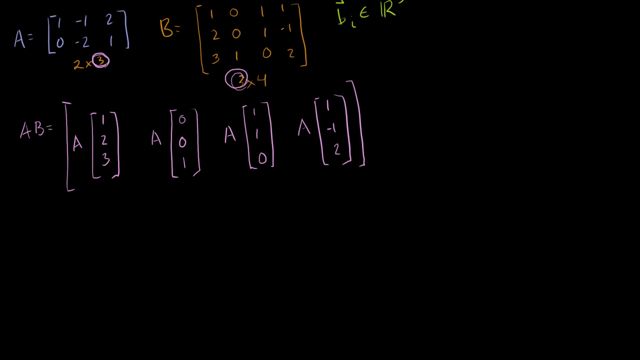 Well, now we've reduced our matrix matrix product problem to just a bunch of four different matrix vector product problems, So we can just multiply these. This is nothing new to us, So let's do it. And so what is this equal to? So AB, let me rewrite it. AB, my product vector, is going to: 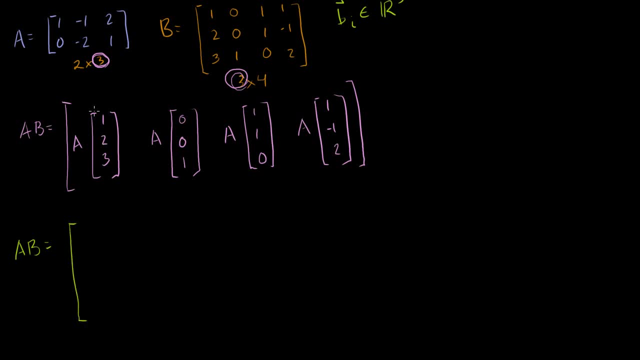 be equal to. so this first column is the matrix A times the column vector 1,, 2,, 3.. And how did we define that, Remember? one way to think about it is that this is equal to the. you can kind of think of it as each of the rows of A. 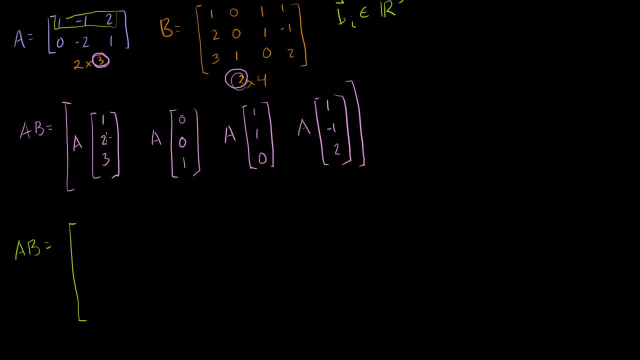 dotted with the column here of B. Or, even better, this is the transpose of some matrix, right, like? let me write this this way: If A is equal to- sorry- the transpose of some vector, let's say that A is equal to the column vector 0, minus 1,. 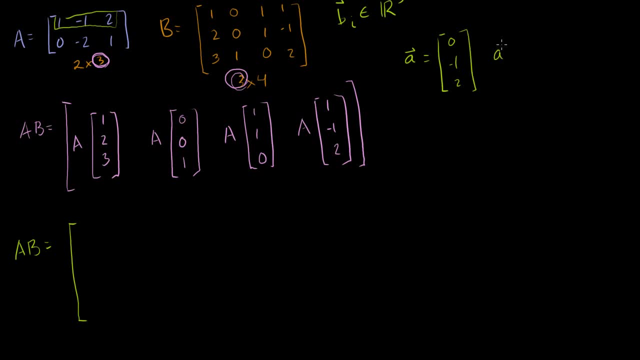 2.. Then A transpose- and I haven't talked about transposes a lot yet, but I think you get the idea. You just change all of the columns into rows, So A transpose will just be equal to 0, minus 1, 2.. 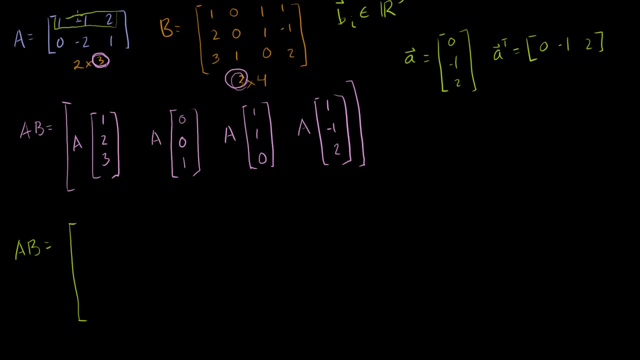 You just go from a column vector to a row vector. So if we call this thing here A transpose, then when we take the product of our matrix, A times this vector, we're essentially just taking the trans. we're just taking A and dotting with this. 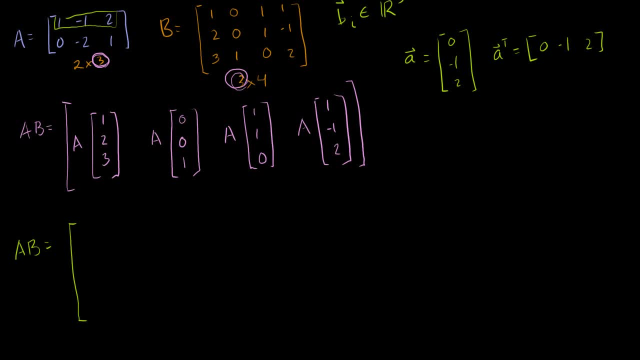 This guy for our first row in our first column. So let me do it that way, So let me write in that notation. So this is going to be the matrix or, sorry, the vector 1, minus 1, 2.. 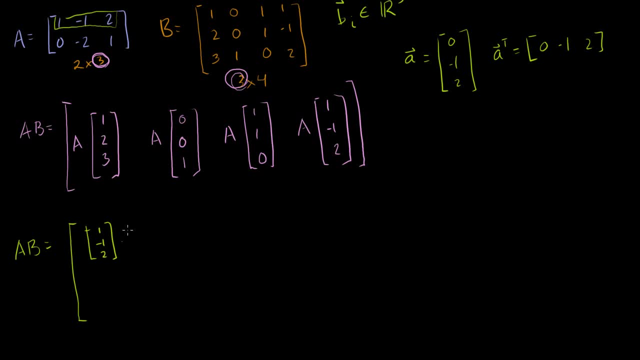 That's essentially that row right there, represented as a column dotted with 1,, 2, 3.. Actually, let me do it in that color, just so I can later switch to one color to make things simple, But dotted with 1,, 2, 3.. 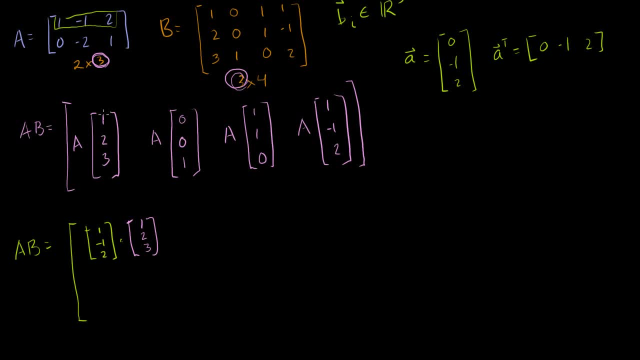 So we just took that row or, I guess, the column equivalent of that row, and dotted with this, And I wrote it like this because we've only defined dot products for column vectors. I could do it maybe for row vectors, but no need to make a. 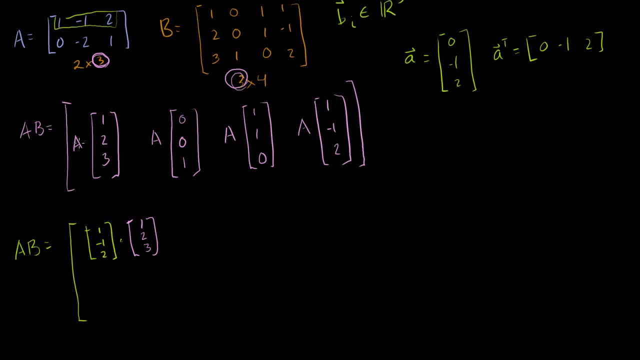 new definition And then the next. so that's going to be the first entry in this matrix vector product. The second entry is going to be the second row of A. The second row of A is essentially dotted with this vector right there, So it's going to be equal to. 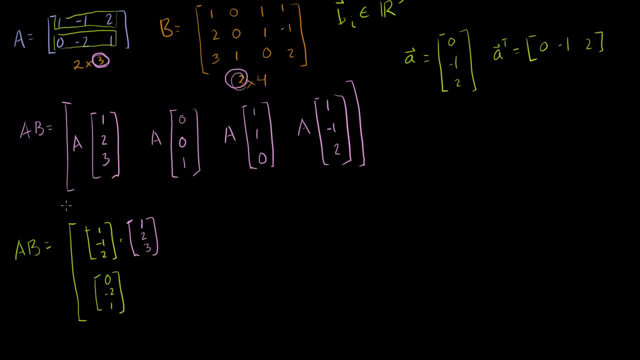 0, minus 2, and 1, dotted with 1,, 2, 3.. Dotted with 1,, 2,, 3.. And we just keep doing that And I'll just switch maybe to one neutral color now. 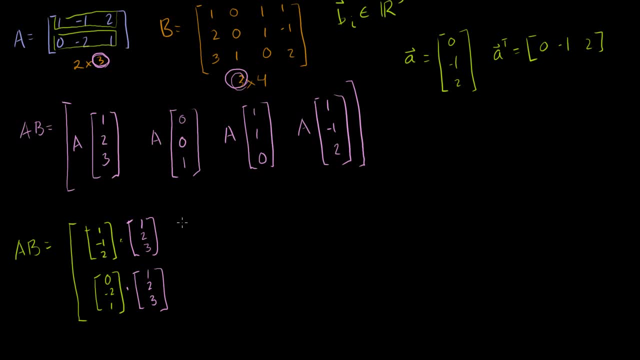 So then, A times 0, 0, 1.. That's going to be the first row of A expressed as a column vector, So we can write it like this: 1, minus 1, 2, dot 0, 0, 1.. 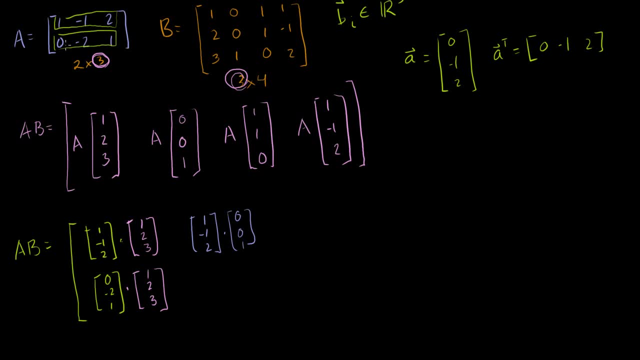 And then Actually, And then we have the second row of A dotted with this column vector. So we have 0, minus 2, 1, dotted with 0, 0, 1.. Two more rows left. This can get a little tedious. 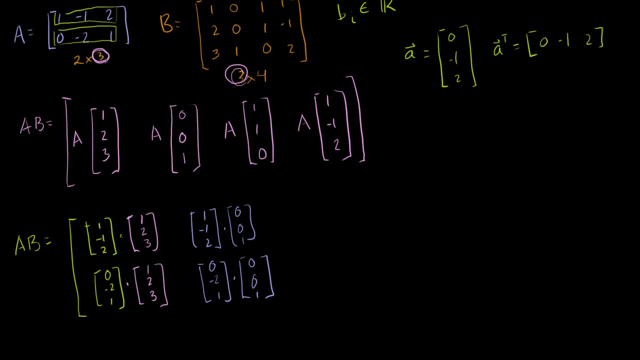 And it's inevitable that I'll probably make a careless mistake. But as long as you understand the process, that's the important thing. The next one: This row of A expressed as a column, vector 1, minus 1, 2.. 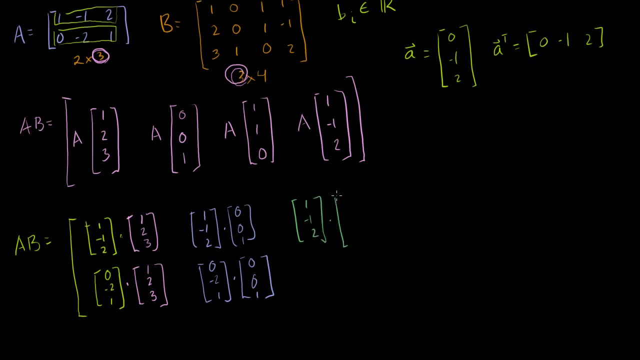 And we're going to dot it with this vector right there: 1, 1, 0.. And then this row of A- I could just look over here as well: 0, minus 2, 1.. Dotted with 1, 1, 0.. 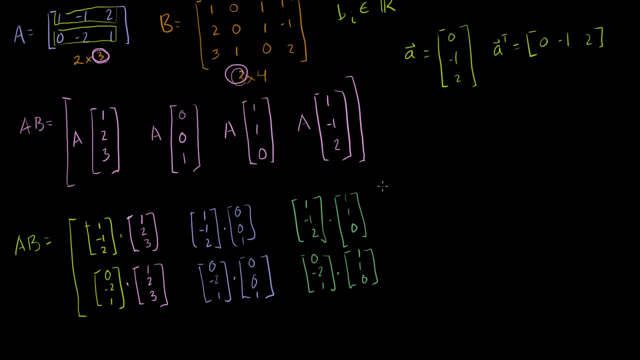 And then, finally, the last two entries are going to be the top row of A: 1, minus 1, 2.. Dotted with this column: vector: 1, minus 1, 2.. A little dot, Remember we're taking the dot product. 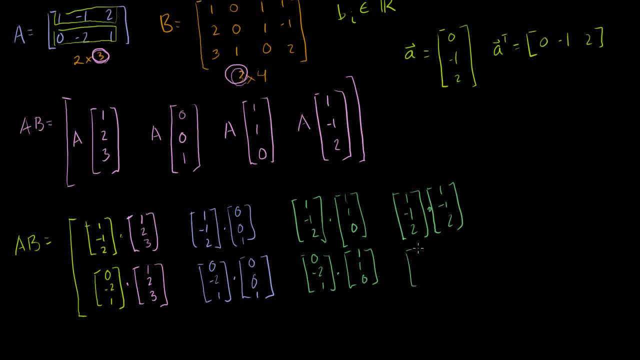 And then, finally, this second row of A, So 0, minus 2, 1.. Dotted with this column, vector 1, minus 1, 2.. And that is going to be our product matrix. And this looks very complicated right now. 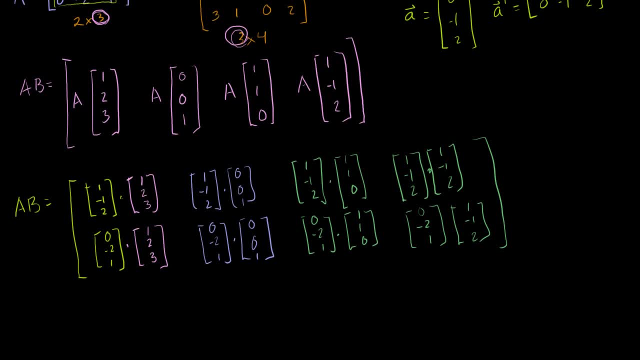 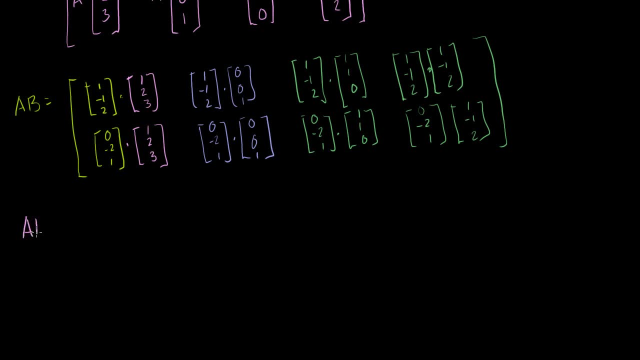 But now we just have to compute it in dot products. Tend to simplify things a good bit. So what is our matrix, our product, going to simplify to? I'll do it in pink. AB is equal to. let me draw the matrix right there. 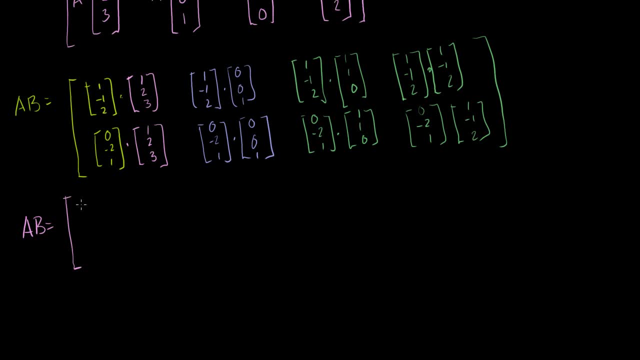 So what's the dot product of these two things? It's 1 times 1.. I'll just write it out: It's 1 times 1.. I'll just write: 1 times 1 is 1. Plus minus 1 times 2.. 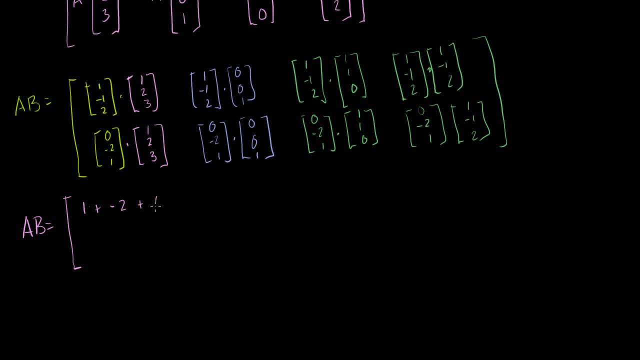 So minus 2.. Plus 2 times 3.. Plus 6.. Now we'll do this term right here: 0 times 1 is 0.. Plus minus 2 times 2.. So that's minus 4.. Plus 1 times 3.. 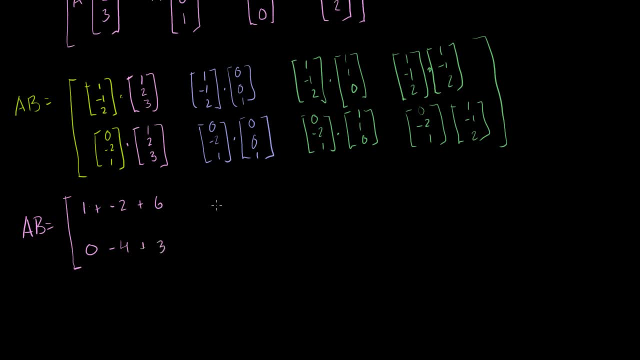 Plus 3.. Now we're on to this term: 1 times 0 is 0.. Plus minus 1 times 0. Plus 0.. Plus 2 times 1 is equal to plus 2.. This term 0 times 0 is 0.. 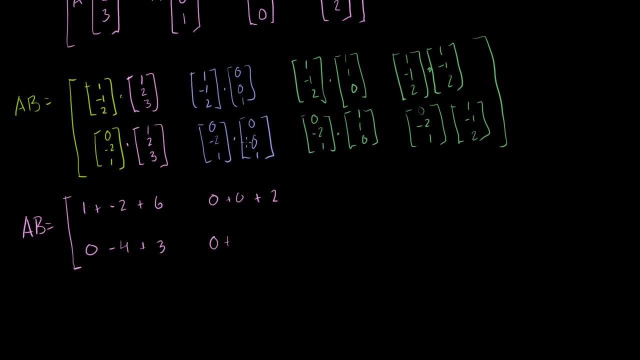 Plus minus 2 times 0, let me write it as 0.. Plus minus 2 times 0 is 0.. Plus 1 times 1.. So plus 1.. Then here you have: 1 times 1 is 1.. 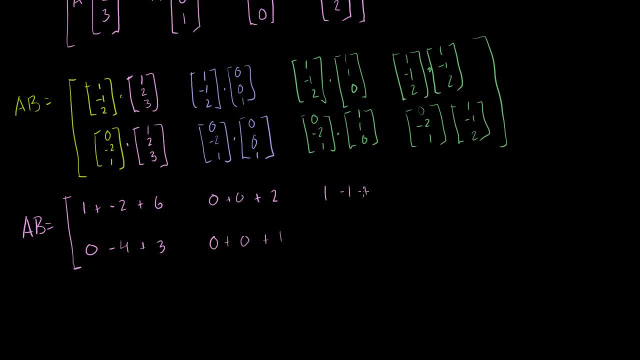 Plus minus 1 times 1 is minus 1.. Plus 2 times 0.. So plus 0.. Here 0 times 1 is 0.. Minus 2 times 1 is minus 2.. And then 1 times 0 is plus 0.. 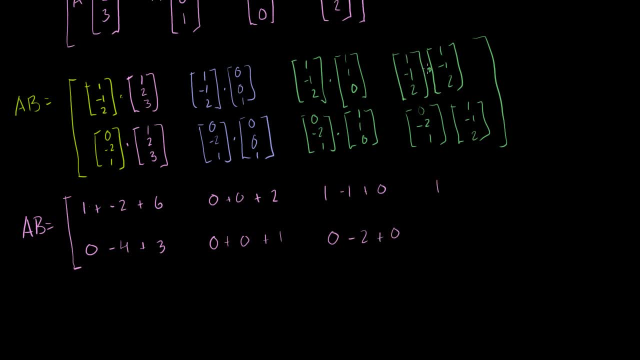 Almost done. 1 times 1 is 1.. Minus 1 times minus 1 is 1.. 2 times 2 is 4.. Finally, 0 times 1 is 0.. Minus 2 times minus 1 is 2.. 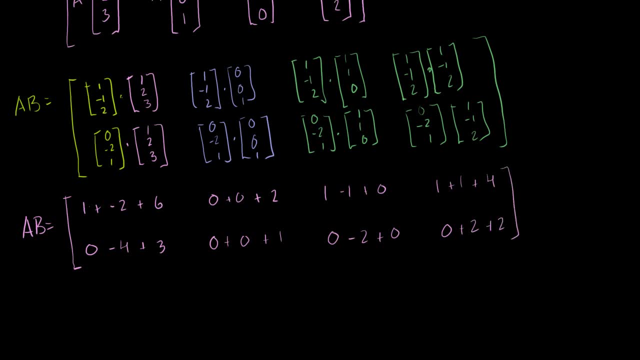 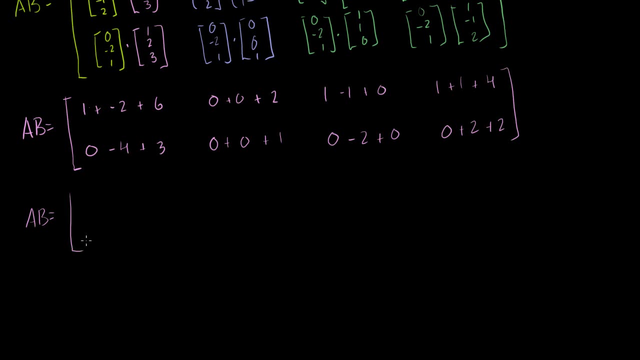 1 times 2 is also 2. And we're in the home stretch. Now we just have to add up these values. So our dot product of the two matrices is equal to the 2 by 4 matrix. 1 minus 2 plus 6, that's equal to 5.. 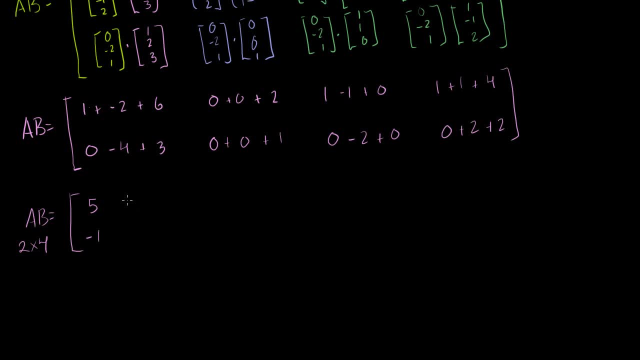 Minus 4 plus 3 is minus 1.. This is just 2.. This is just 1.. Then we have 1 minus 1 plus 0 is just 0.. Minus 2. We just have a minus 2 there. 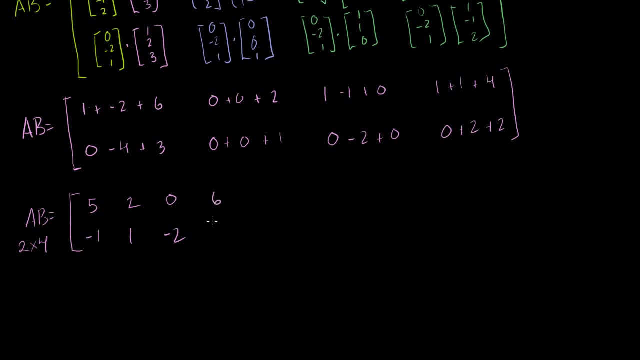 1 plus 1 plus 4 is 6.. And then 2.. And then 2 plus 2 is 4.. And we are done. The product of AB is equal to this matrix, right here, And let me get my A and B back. 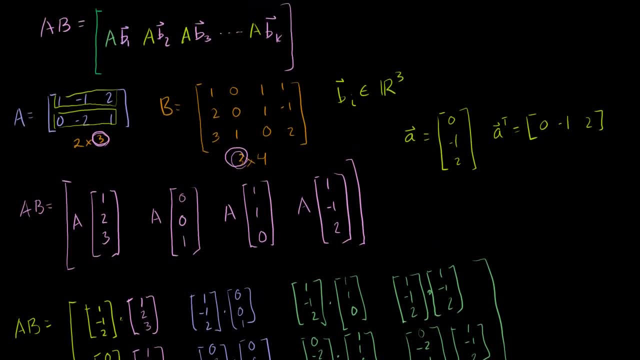 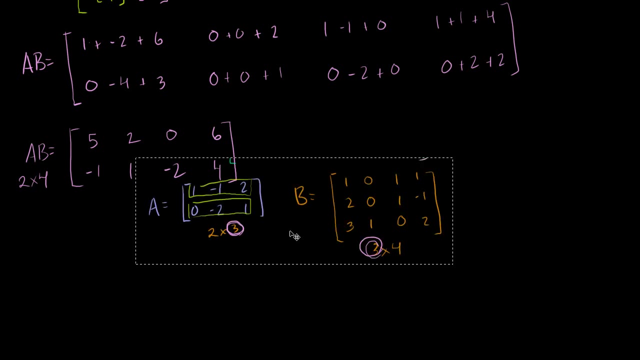 We can talk a little bit more about what this product actually represented. So let me copy and paste this And then I'll paste it. Let me scroll down a little bit, Go down here, Paste, There you go. So this was our A and our B. 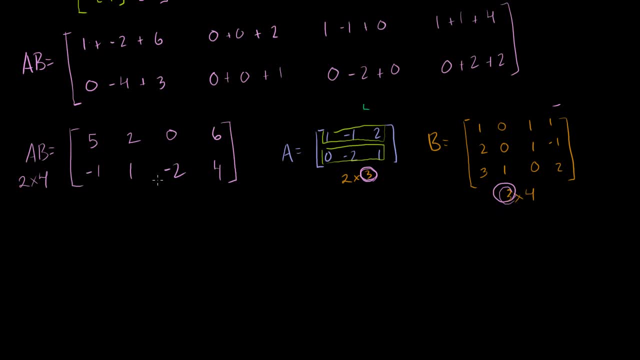 OK, OK, And when we took the product, we got this matrix here. Now there are a couple of interesting things to notice. Remember, I said that this product is only well-defined when the number of columns in A is equal to the number of. 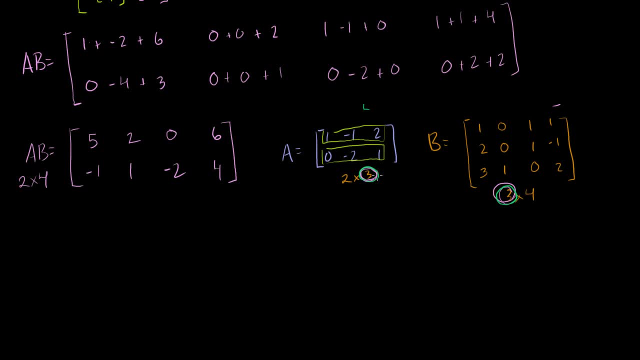 rows in B. So that was the case in this situation. And then notice we got a 2 by 4 matrix, which is the number of rows in A times the number of columns in B. So we got a 2 by 4 matrix. 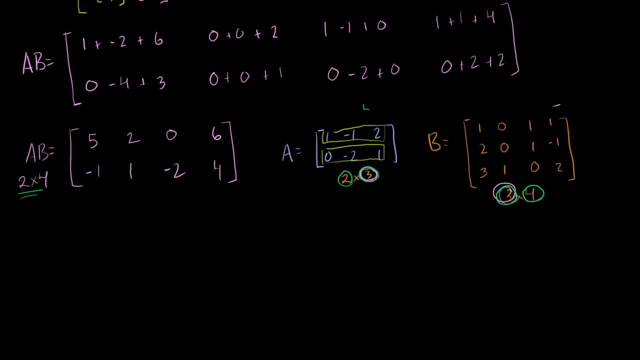 So another natural question Is: could we have found, or is it even equal, if we were to take the product BA, If we were to even take the product BA? So if we tried to apply our definition there, what would it be equal to? 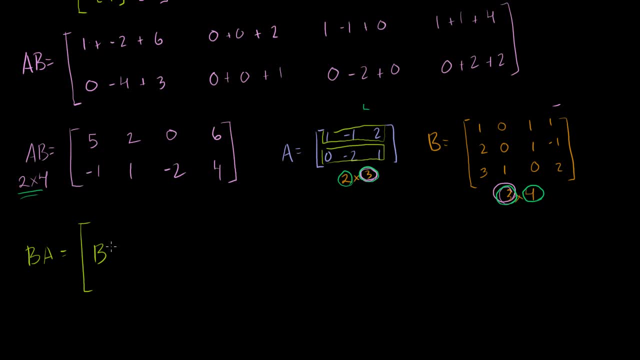 It would be equal to the matrix B times the column 1, 0. Then the matrix B times the column minus 1, minus 2.. And then it would be the matrix B times the column 2, 1.. Now, 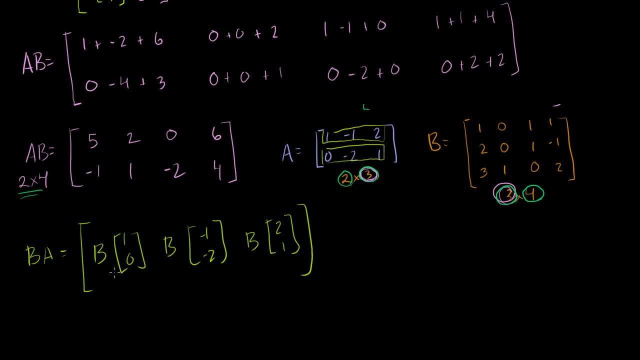 Can we take this matrix vector product? We have a 3 by 4.. This right here is a 3 by 4 matrix And this guy right here is a member of R2.. So this is not well-defined. We have more columns here than entries here. 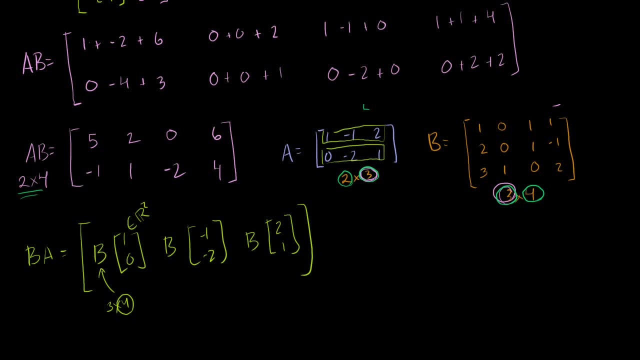 So we have never defined a matrix vector product like this. So not only is this not equal to this, it's not even defined. So it's not defined When you take a 3 by 4 matrix And you take the product of that with a 2 by 4 matrix. 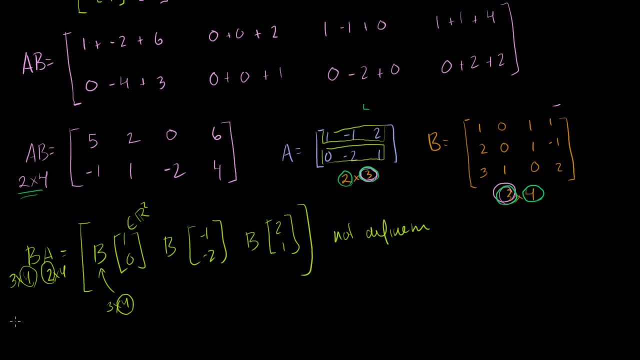 It's not defined because that number and that number is not equal. And so, obviously, since this is defined and this isn't defined, you know that AB is not always equal to BA. In fact, it's not usually equal to BA And sometimes it's not even defined. 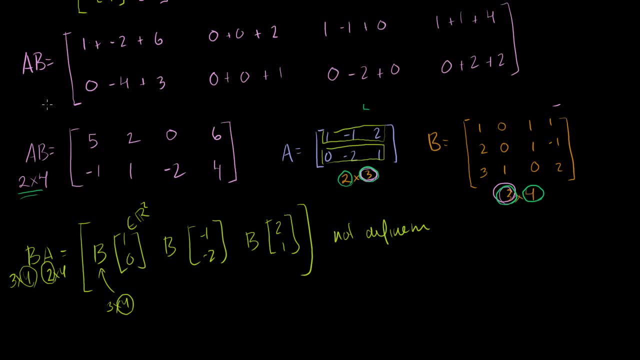 And the last point I want to make is: you probably learned to do matrix- matrix products- in Algebra 2, but you didn't have any motivation for what you were doing. But now we do have a motivation Because when you're taking the product of A and B, we 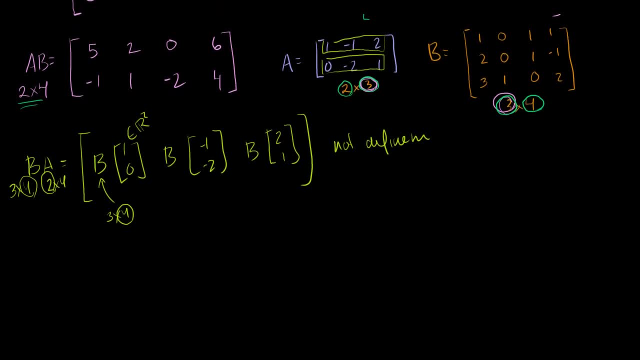 learned in the last video that if we have two transformations, Let's say we have the transformation S is a transformation from R3 to R2.. And that S is represented by the matrix. So S given some matrix in R3, if you apply the. 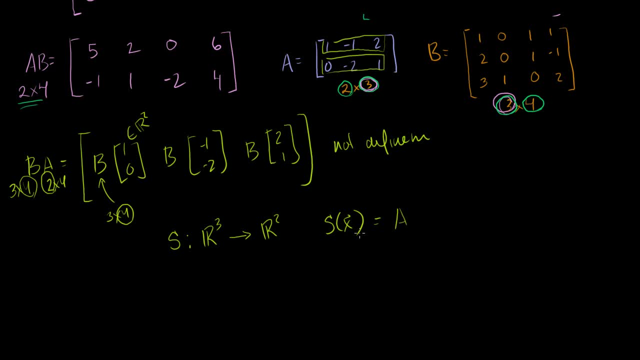 transformation S to it, it's equivalent to multiplying that. or given any vector in R3, applying the transformation S is equivalent to multiplying that vector times A. We can say that, And I used R3 and R2 because the number of columns in A is. 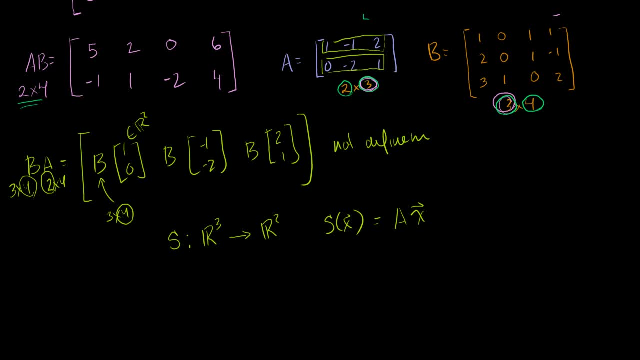 3, so it can apply to a three-dimensional vector. And similarly we can imagine B as being the matrix transformation of some transformation T. that is, a mapping from R4 to R3, where if you give it some vector x in R4, it will produce. you take the product of that with. 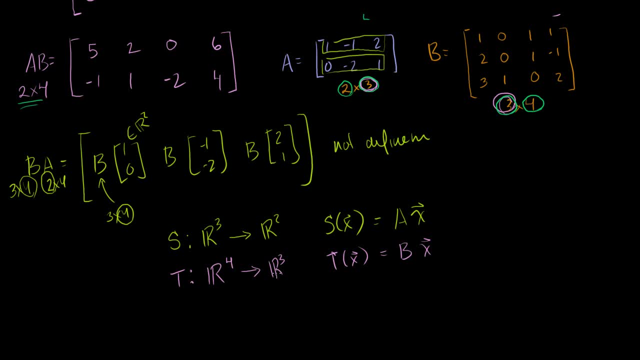 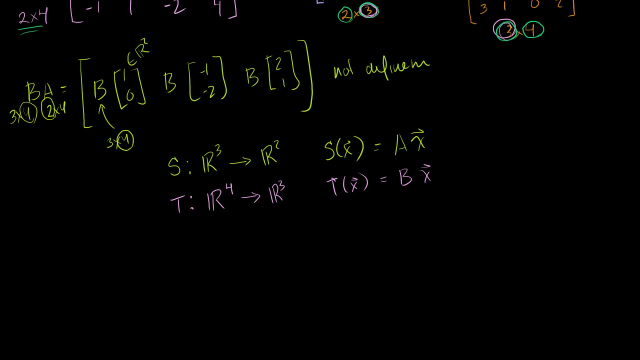 B and you're going to get some vector in R3.. Now, if we think of the composition of the two, so let's think about it A little bit. If we have R4 here, let me switch colors. We have R4 here. 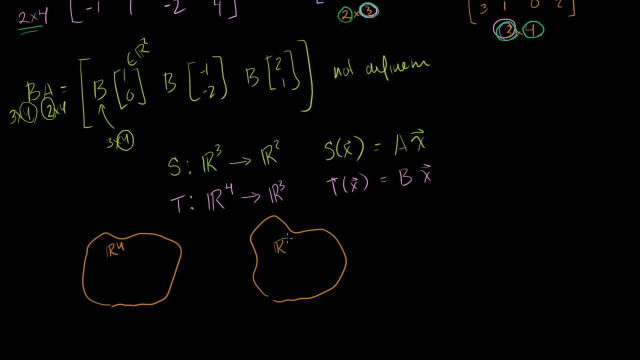 We have R3 here And then we have R2 here. T is a transformation from R4 to R3.. So T will look like that. T is a transformation. It's B times x. That's what T is equal to. 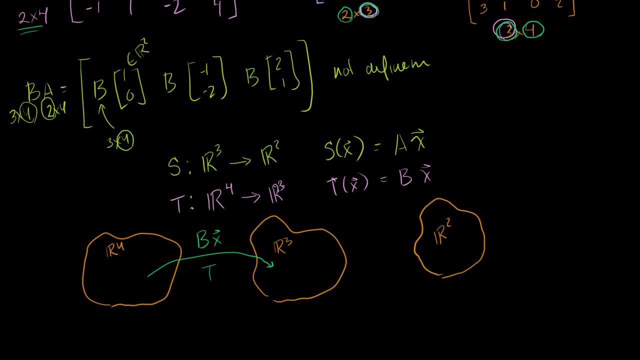 So T is this transformation And then S is a transformation from R3 to R2.. So S looks like that And S is equivalent to A times any vector in R3.. So that is S. So now we know how to visualize, or how to think about what the 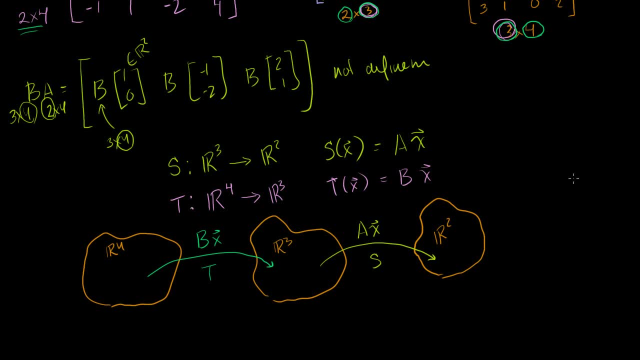 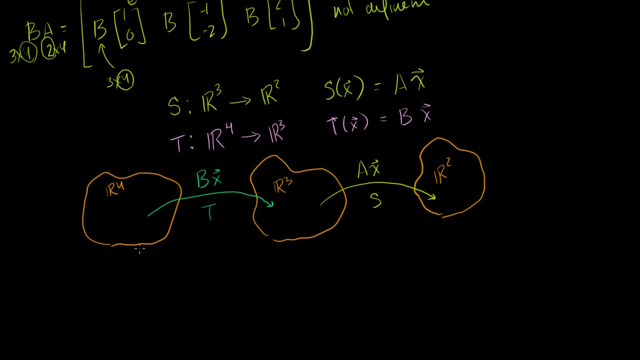 product of A and B are. The product of A and B is essentially, you apply the transformation B first. So let me think of the composition of S. Let me write it this way. So what is the composition of S with T? This is equal to of x. 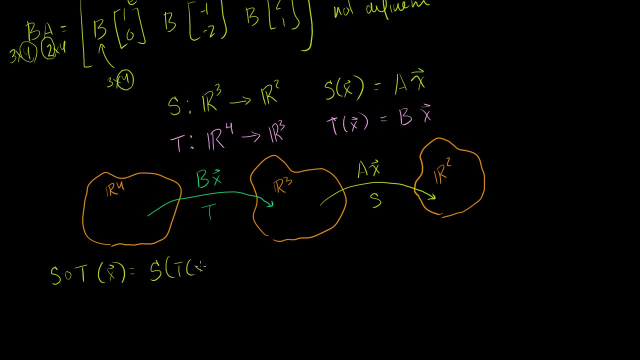 This is equal to S of T of x. So you take a transformation from R4 to R3, and then you take the S transformation from R3 to R2.. So this is S of 3.. S of T is a transformation from R4 all the way to R2.. 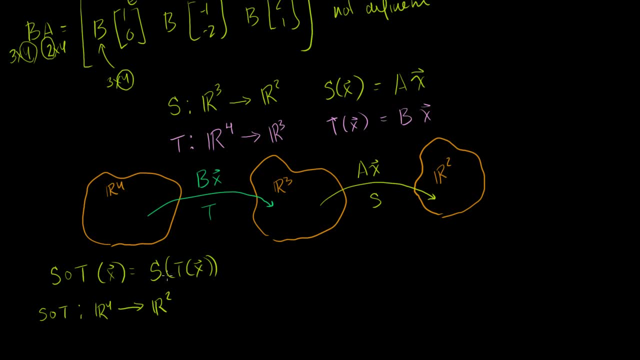 And then the neat thing about this: if you were to just write this out in its matrix representations- we did this in the last video- this would be equal to the S matrix A times this vector right here, which is Bx. But now we know that the matrix, by our definition, of 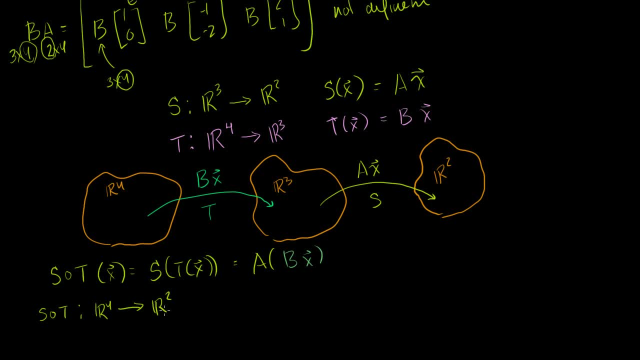 matrix vector products. This guy right here is going to have a transformation. It's going to be equal to the composition s of t of x, is going to be equal to the matrix AB, based on our definition. so the transformation AB times some. 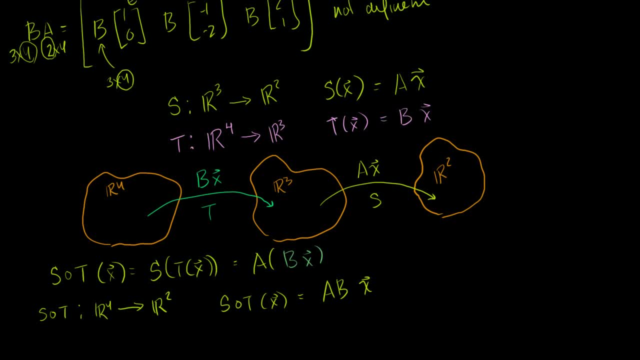 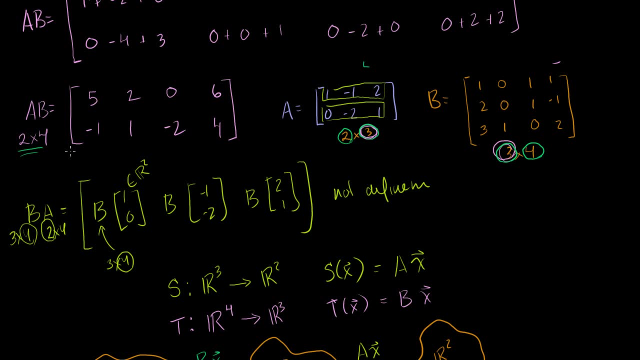 vector x. So the reason why I'm going all of this is because we just did a matrix product up here. We took the pain of multiplying the matrix A times the matrix B and we got this value here And hopefully I didn't make any careless mistakes. 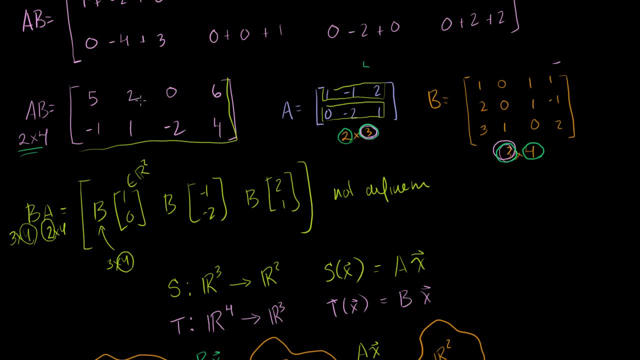 But the big idea here, the idea that you probably weren't exposed to in your Algebra 2 class, is that this is the matrix of the composition of the transformations s and t. So right here it's the matrix of the composition of s and t. 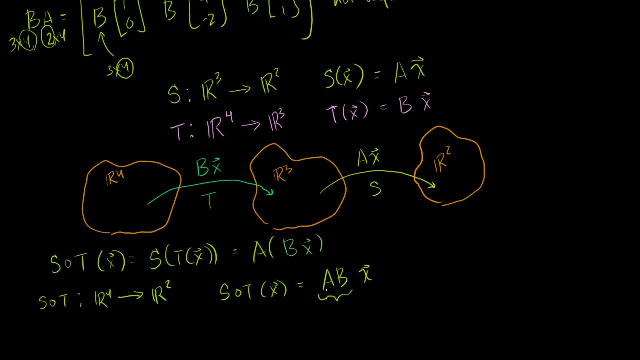 So you're not just blindly doing some matrix. matrix products can be pretty tedious, But now you know what they're for. They're actually for the composition of two transformations, where each of A and B are the transformation matrices for each of the individual linear.